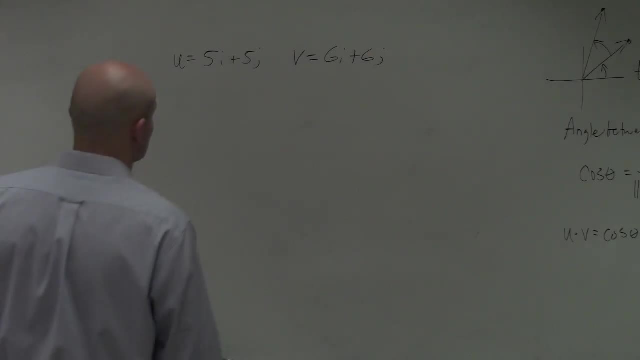 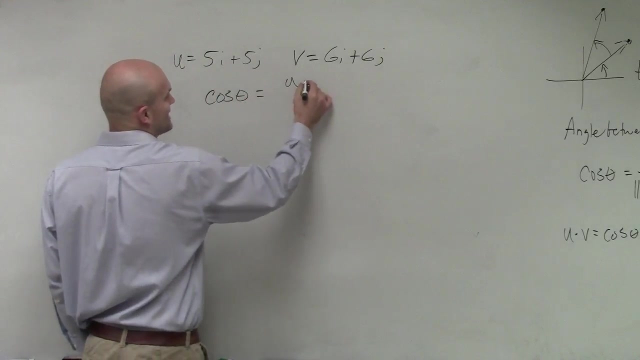 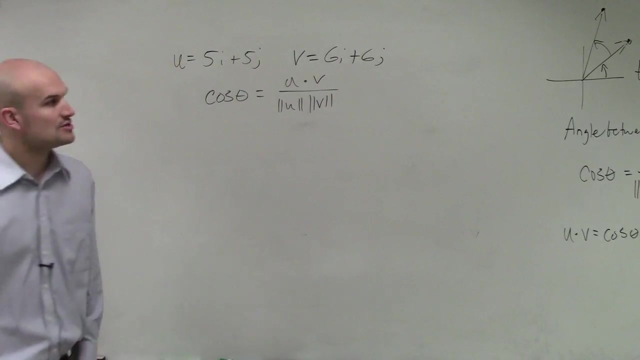 The angle between these 2 vectors. So remember, the angle between these 2 vectors is going to be: cosine of theta equals the dot product of the magnitude of u times the magnitude of v. so what I'm gonna do is I'm just gonna work on this and let's just, we know we have. 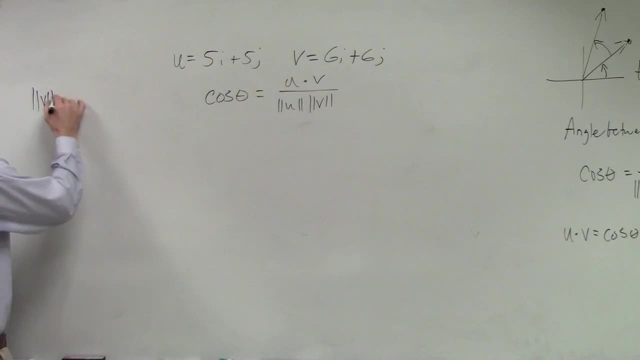 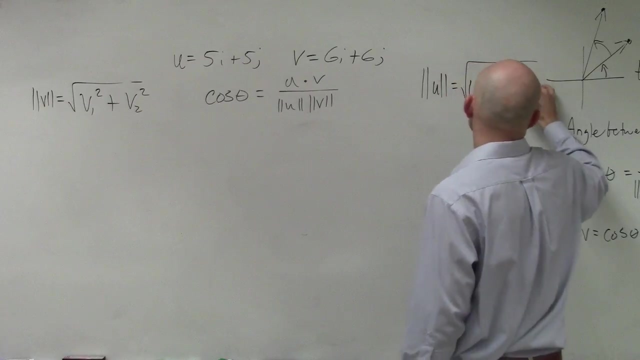 to find the magnitudes. so let's do. the magnitude of v equals the square root of v1 squared plus V2 squared, And the magnitude of U equals the square root of U1 squared plus U2 squared. right Definition of magnitude. We've got to make sure we know those and go through it. 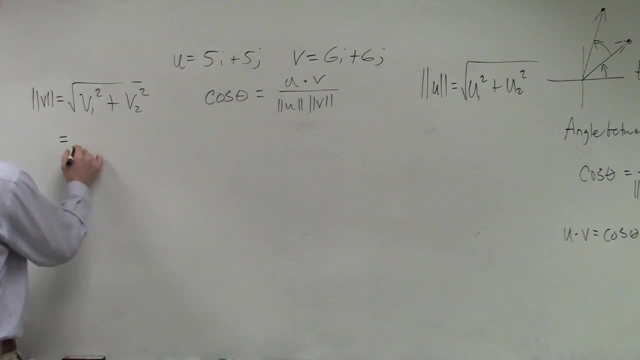 So here this is going to equal square root of, so we'll have 5 squared plus 5 squared. 25 plus 25 is the square root of 50, which I can reduce to 5 radical 2,. right Over here I have 6 squared. 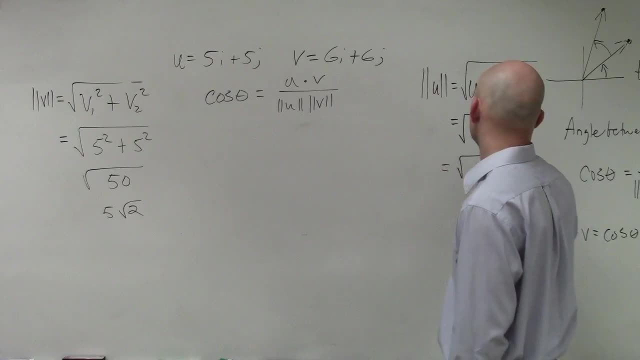 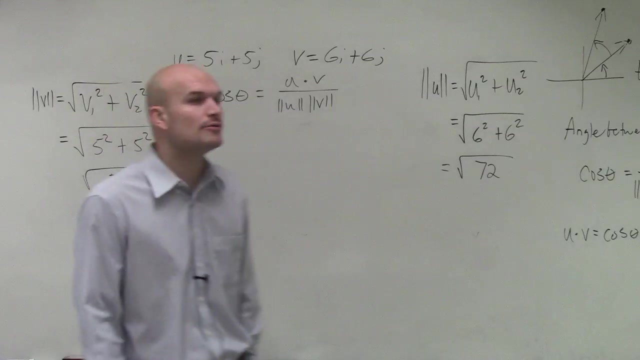 plus 6 squared, which is going to be 72.. Okay, So you take square root of 50 and you say what is the largest number That I can take the square root of, that I can write as a product in 50.. Well, you look at 4.. 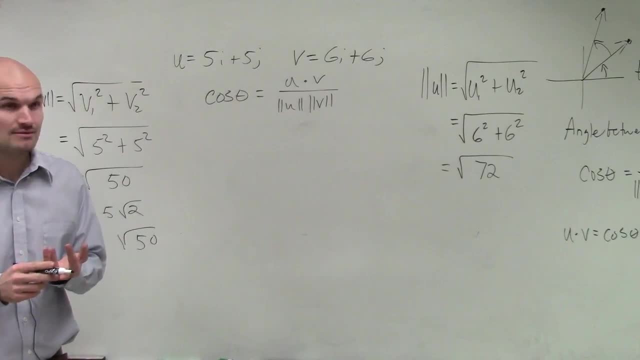 Does 4 divide into 50? No, You take 9.. Does 9 divide into 50? No, You take 16.. Does 16 divide into 50? No, Then you go to 25.. Does 25 divide into 50? Yes, So you just rewrite it as 25 times. 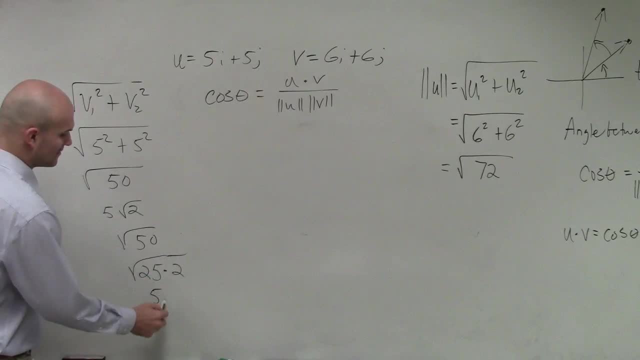 2. What's the square root of 25? 5. Can't take the square root of 2, so you leave it out there. So it's 5 squared of 2.. Okay, Was it were? you just telling me the answer. 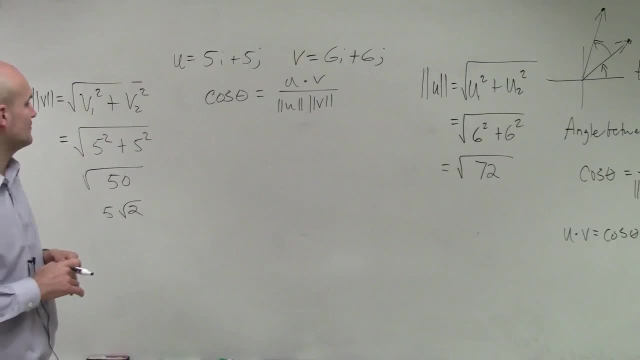 No for v, it's negative 6: 1. v is negative 6. Here, Yeah, Oh really No, it's not, Yeah, it's negative 6. It's yeah, I mean I, I mean, I could say that. 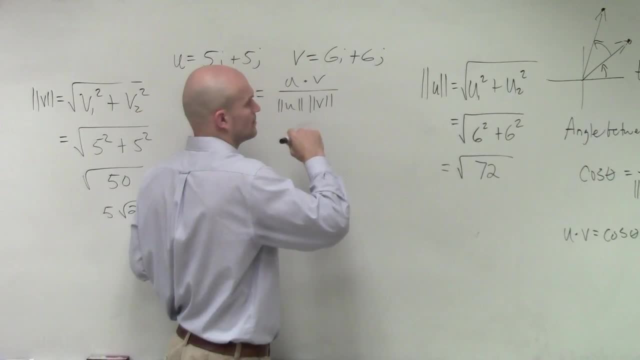 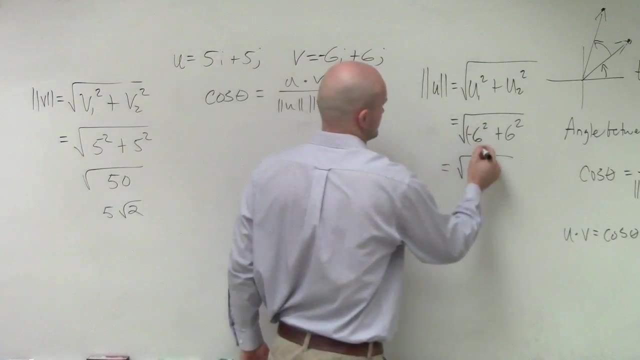 Yeah, but you could do when you square it. it's going to be positive, i, It's negative. 6 i Okay, This would still be the same number. Yeah, Okay, Thank you. So we have 5 squared. 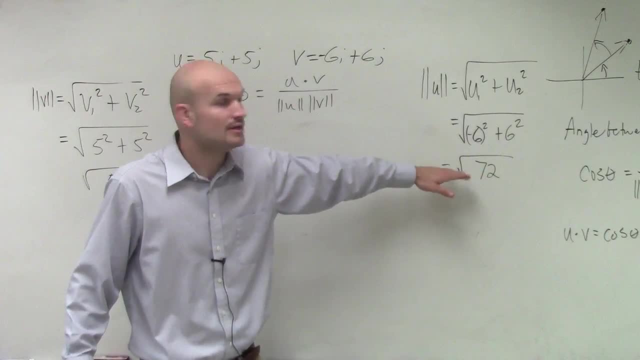 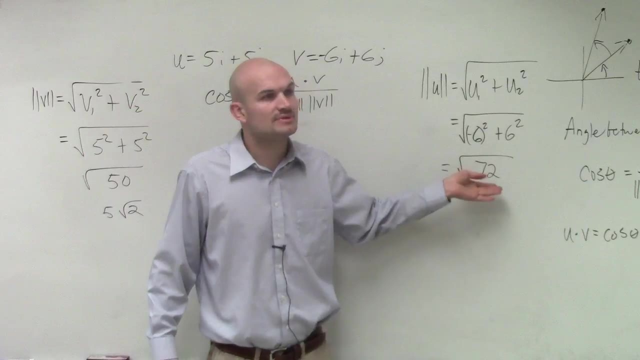 5 squared of 2.. Here we still get 72.. So now let's go back through it again. Does 4 divide into 72?? Yes, it does, But let's see if there's a higher one, right? What about 9?? Does 9 divide into there? 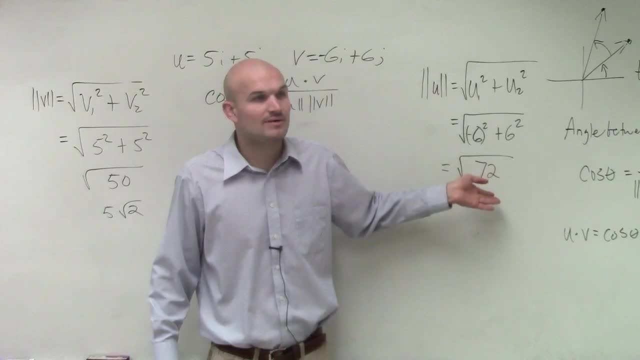 Yes, it does. Let's see again. Is there a higher one? What about 16?? 16 would give you 32, would give you 64.. And if you had 16 again, what would you do? No, No. 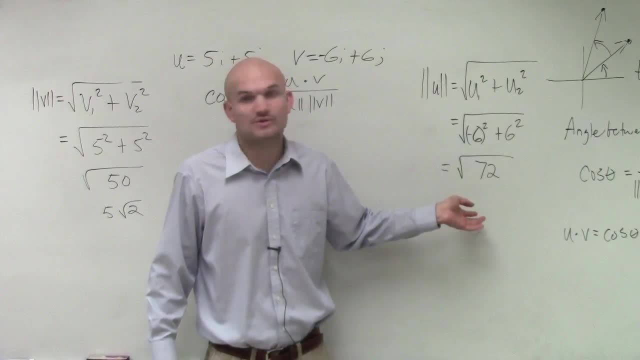 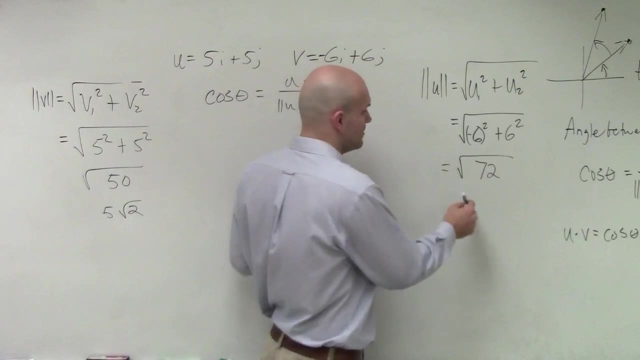 No, No, Okay. So 16 doesn't work. How about 25?? Does 25?? No, No. What about 36?? Yes, Yeah. So you could have done 4.. You could have done 9.. But you always want to choose. 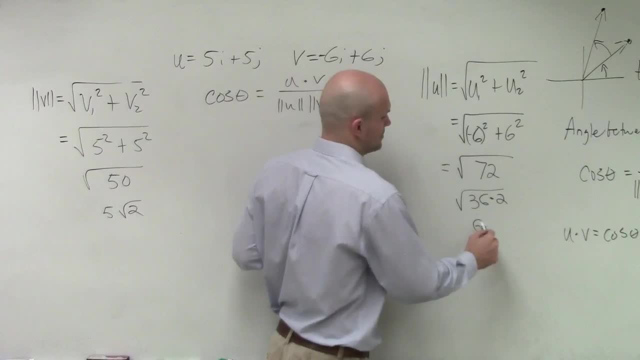 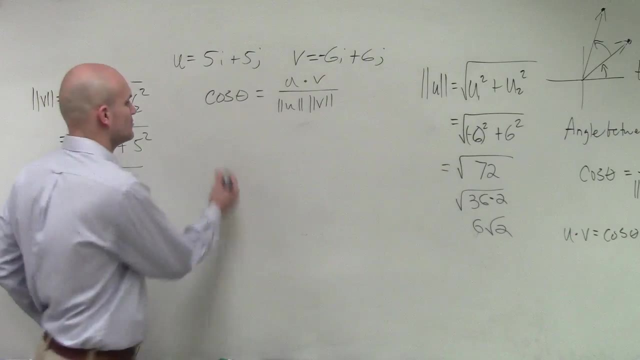 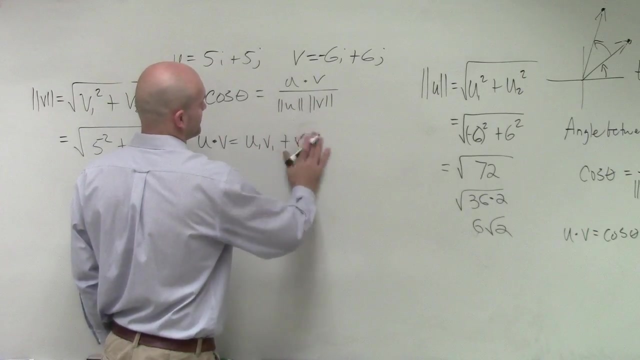 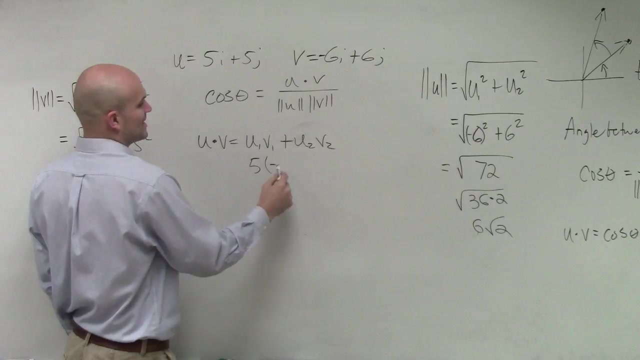 the largest number that divides in Asking for the number. Okay, So now we need to do the dot product. Remember the dot product. u dot v equals u1 times v1 plus u2 times v2, right? So therefore we go through this. It's 5 times negative. 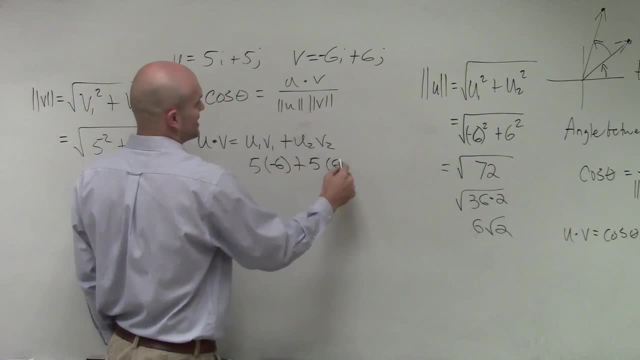 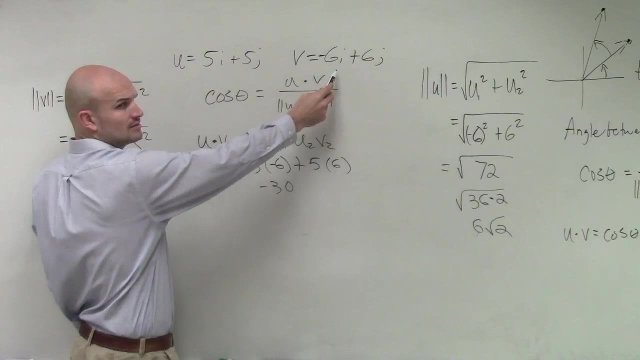 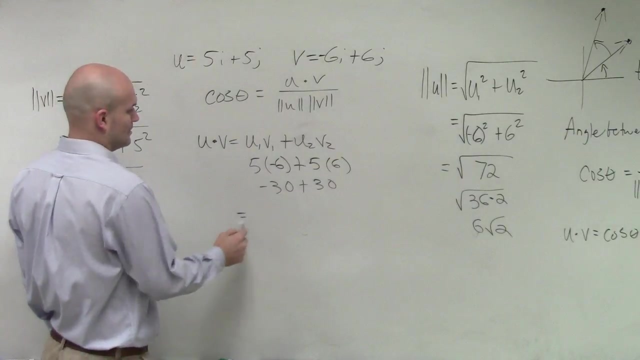 6 plus 5 times 6.. So therefore, this equals negative 30.. Is this right? Yes, Okay, Negative 30 plus 30. Well, therefore, Negative 31.. Negative 30 plus 31.. Negative 31.. 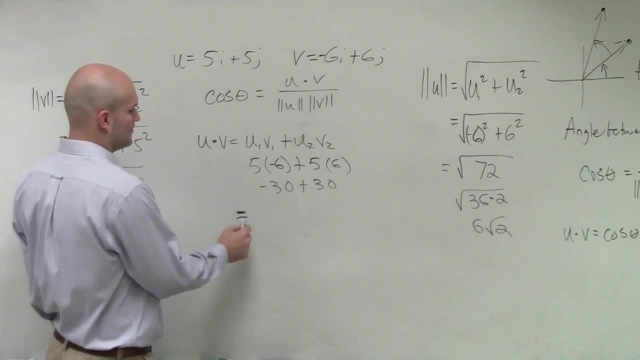 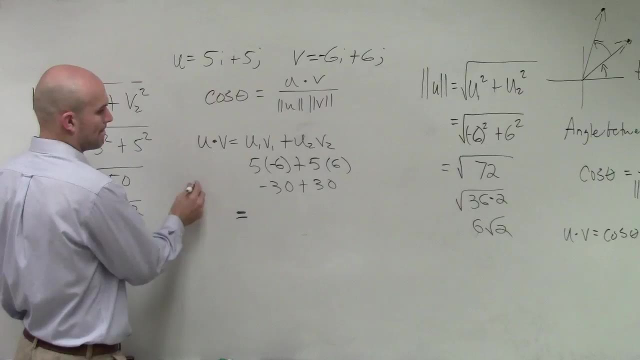 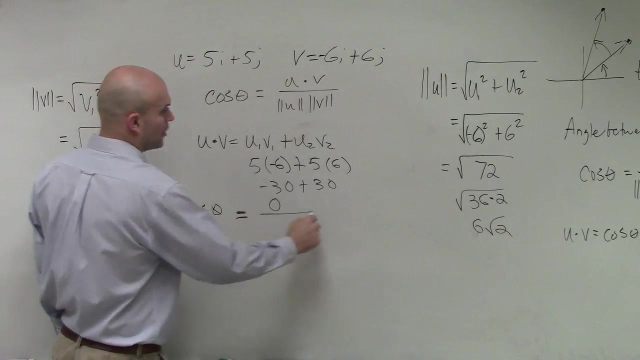 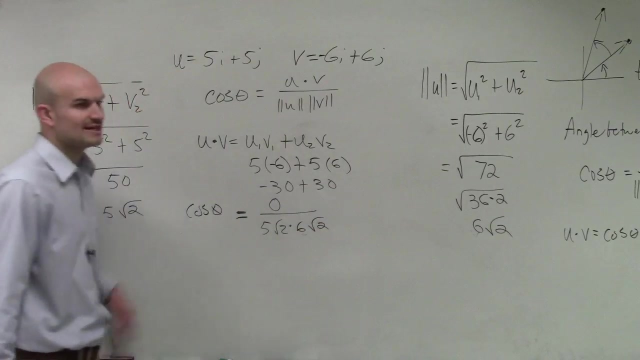 Negative, 31.. Negative, 31.. So if you guys have it on 0, what am I looking at? Okay, So therefore I'm going to have 0.. So I have: cosine of theta equals 0 over 5 square root of 2 times 6 square root of 2.. Now, obviously, guys, you can reduce. 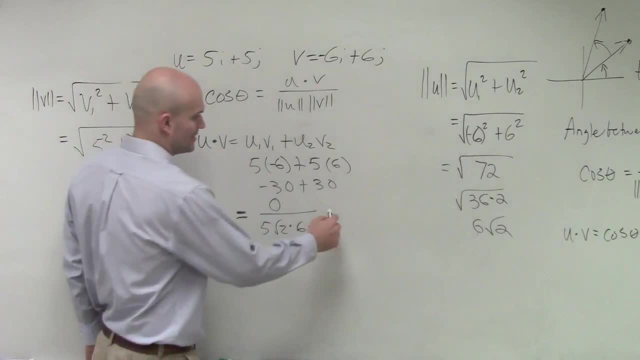 this to 30 times 2,, which would be 2, right. 0.. 0 over 60, right. But we know this is pretty much a waste of time because we know it doesn't really matter what I have in the denominator. I have 0. 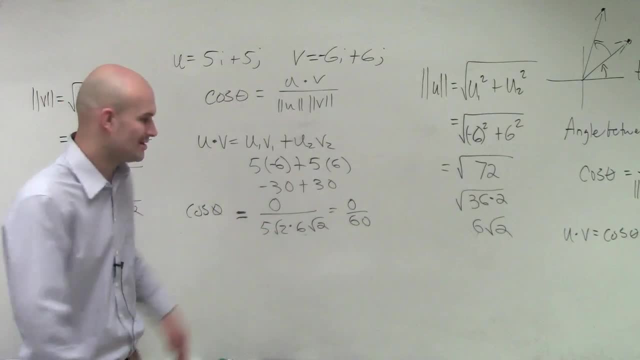 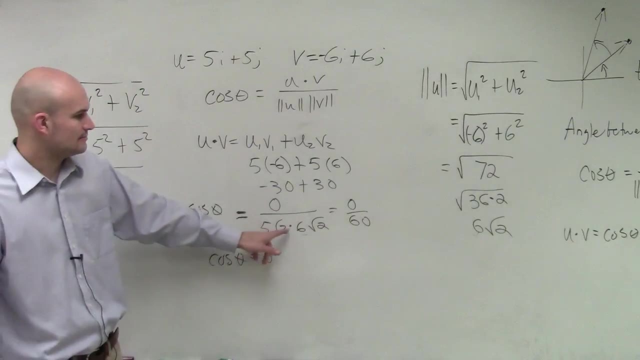 in the numerator, so my answer is going to be 0.. Oh, so those 2's make 2, and then 5 times 6 is 30 times another 2.. But in this case it's not going to affect our answer. Cosine theta equals.